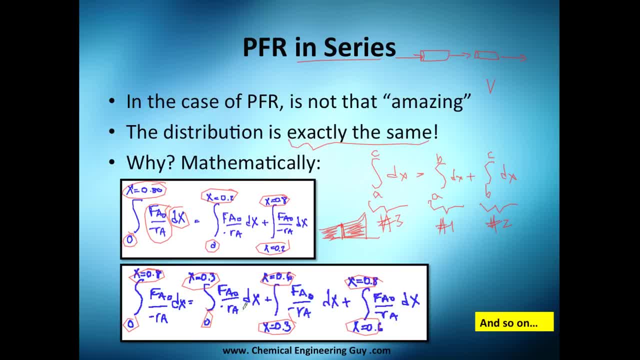 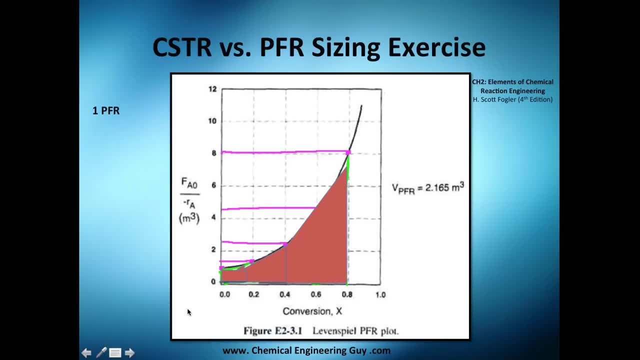 And what did I just do is I got three reactors, but I'm having the same volume as if I will have one reactor. So you can see it more graphically. It's not that impressive. I tell you, this is one reactor. You have all the area under this curve. Now this will be two. 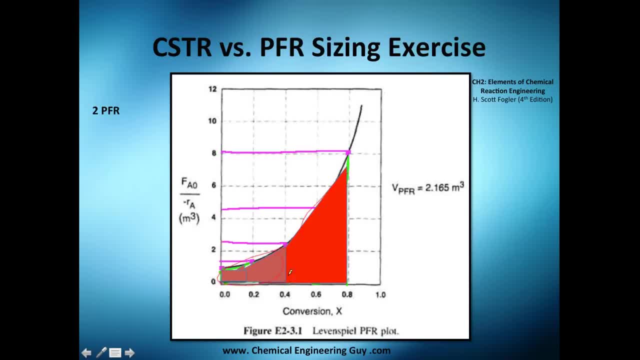 reactors, This area and this area here, or three reactors, We are still speaking about the same total value, which is this one. So you can have as many PFRs you want and you will still have the same value. So why would you do that? You don't need to do that, Maybe because you have not. 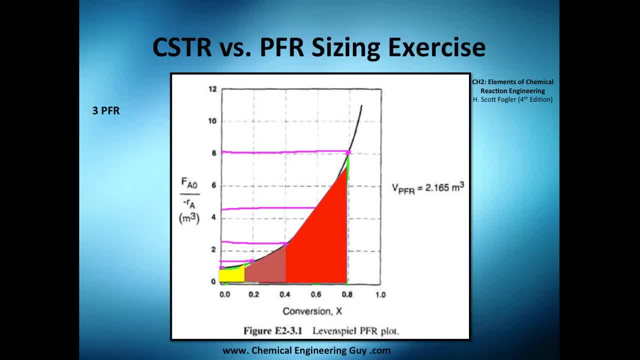 space, Not that much space You don't want to. Maybe you want to do one in one room and the other in one room so you can analyze them, or maybe you don't like working with huge units. Whatever the case, the volume is going to be the same. 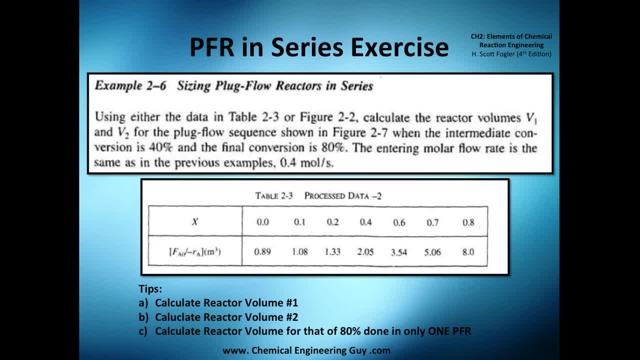 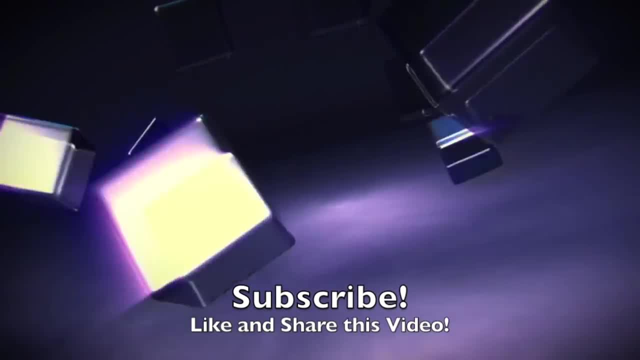 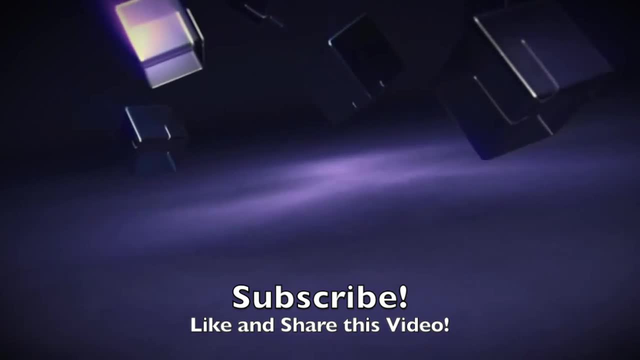 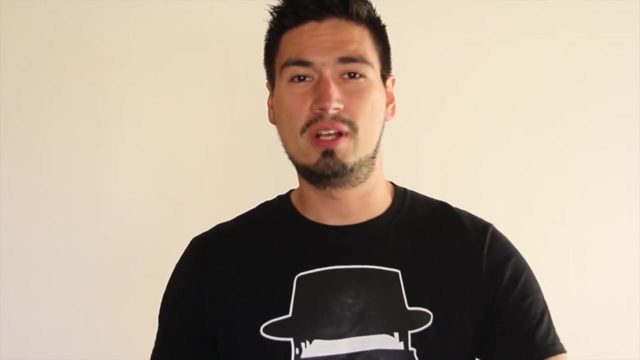 And I bring you this exercise, but I'm going to drop it for the next video. What's up guys? It's me Chemical Engineering Guy. So if you liked the video, why not push the like button? It really helps me to know if you're liking the videos or if I should be. 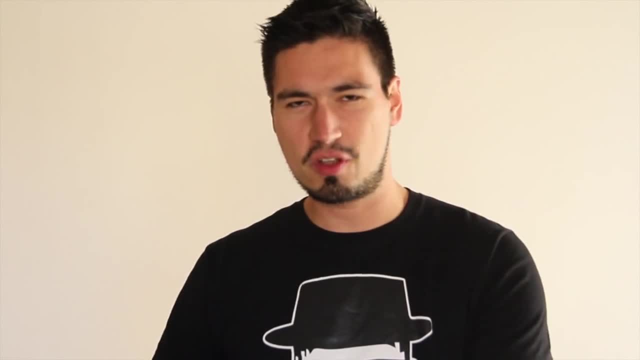 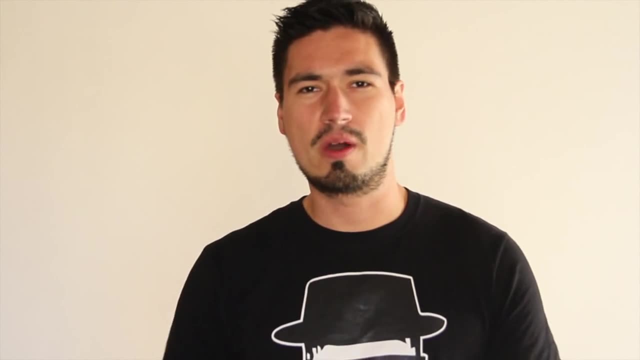 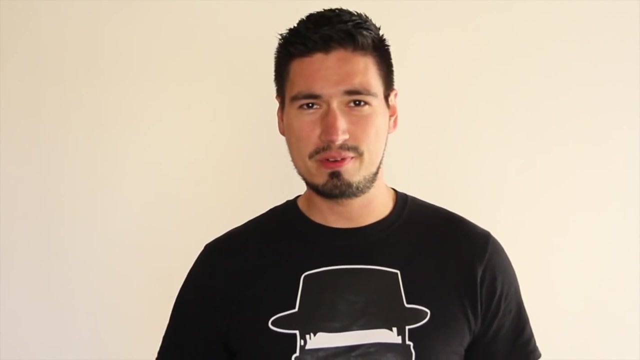 changing something, or I should be adding something, taking out content whatever. Also, sharing is caring, So if you got any kind of friends, teachers, colleagues or whatever kind of person that might be interested in this type of content, why not share it? Sharing helps our community to grow faster in members. 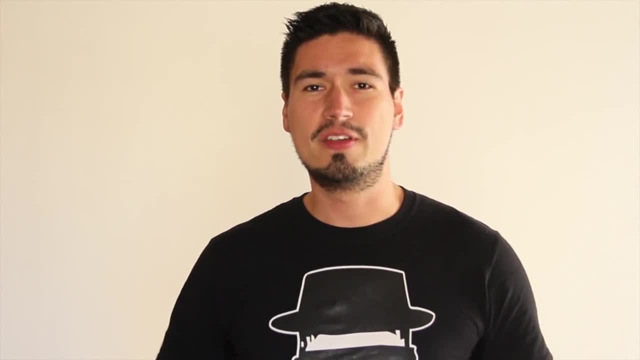 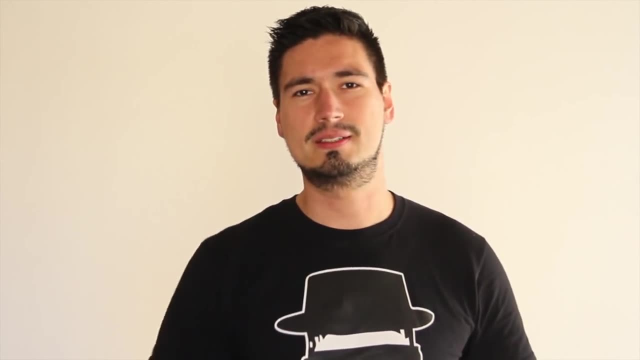 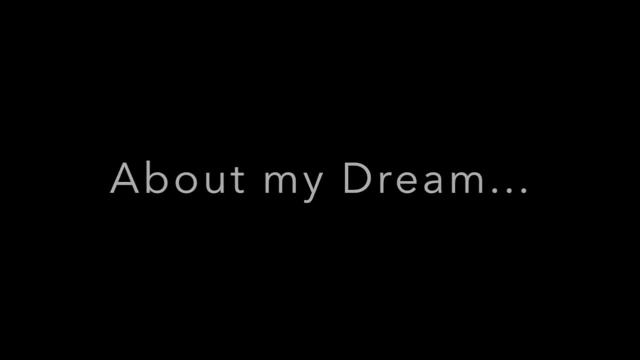 and in content. If you want to keep track of my activity, videos, uploads, experiments, playlists, whatever content I'm getting on YouTube, be sure to click the subscribe button. Subscribing to the channel is totally free, guys. My dream is to create an online Academy of Chemical Engineering where everyone 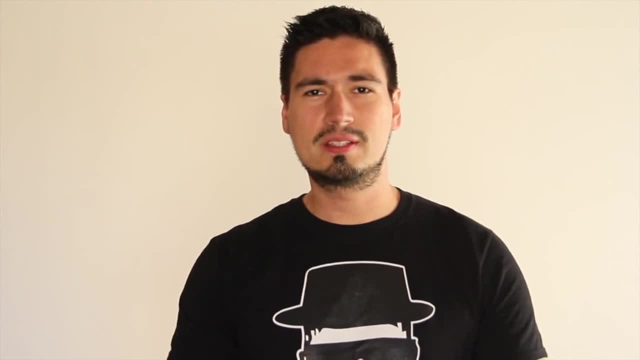 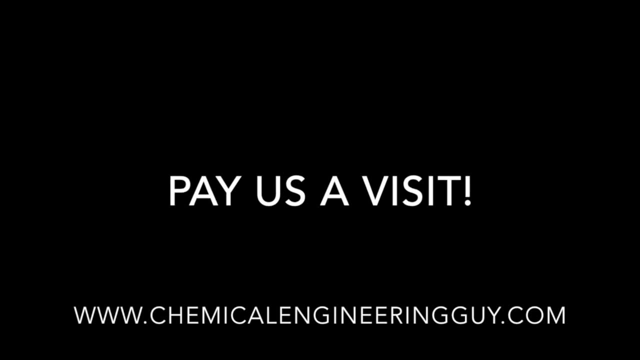 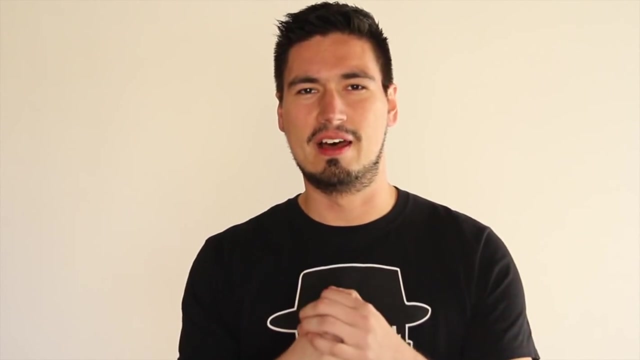 can access it in the world. Imagine a place in which the student, the teacher and the engineer get the best of each other. Thank you, thank you, thank you, guys, for the support and the love.